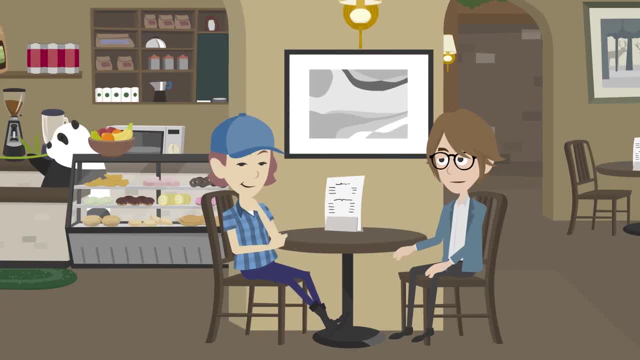 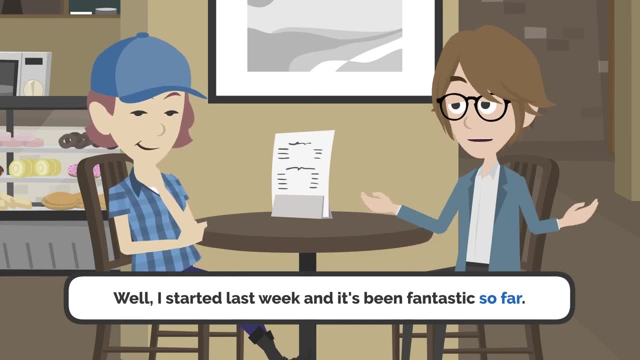 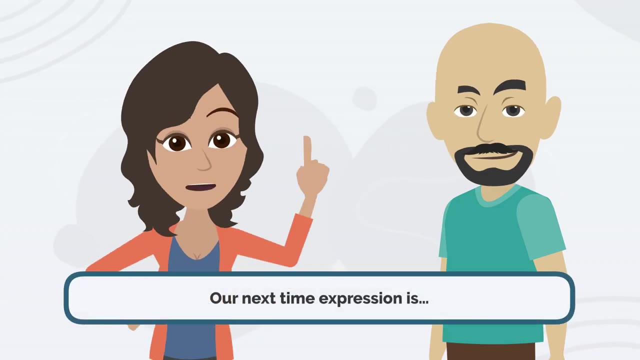 It's used with present perfect tense: How is your new job going Well? I started last week and it's been fantastic so far. I'm enjoying the work and getting along well with my colleagues. Our next time expression is: Oh, the cat needs attention. I will be right back. 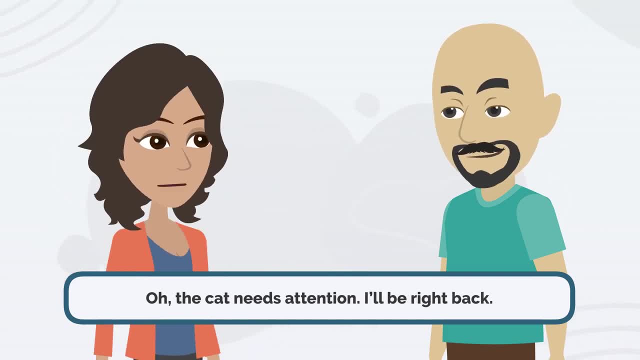 Okay, In the meantime, I'll continue our video. The next time expression is In the meantime. We use this to say what we will do or what will happen while we wait for something else to happen. You can also say meanwhile. They mean the same thing. 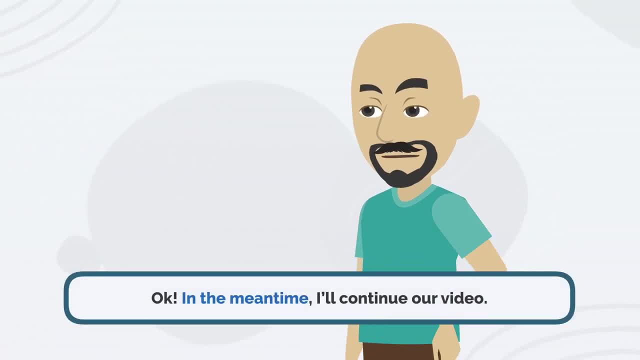 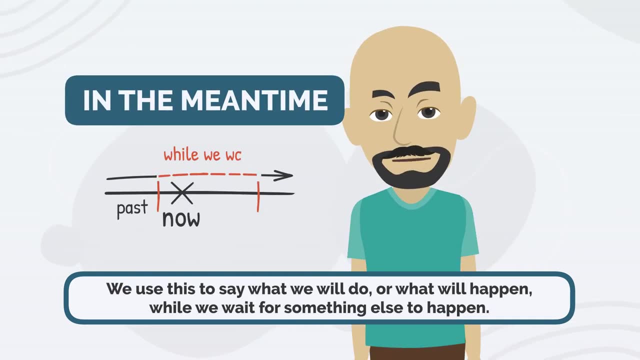 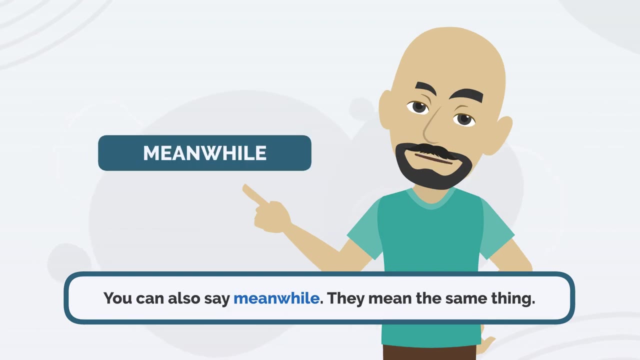 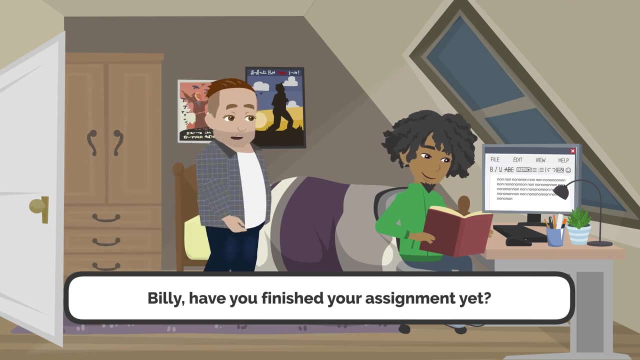 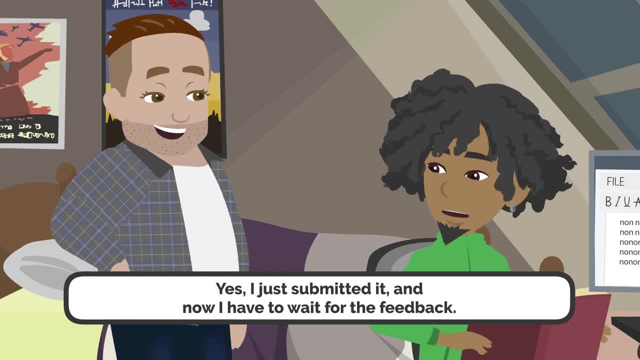 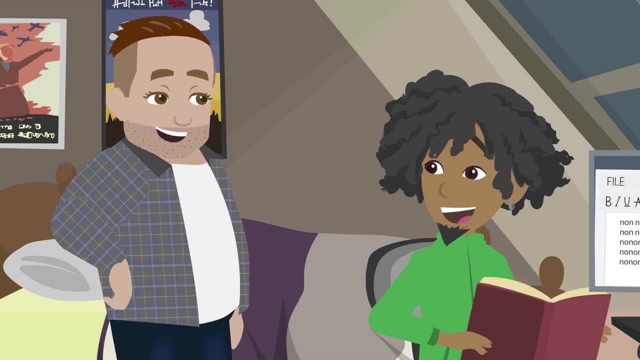 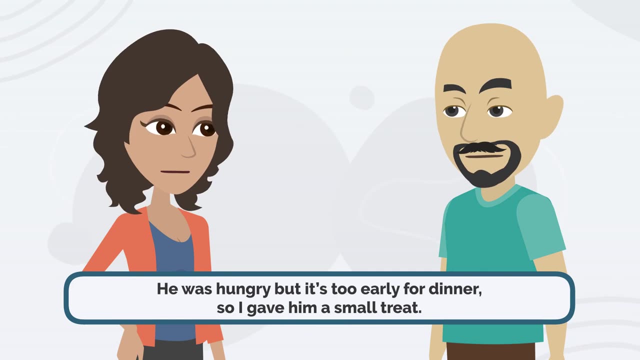 Yes, I just submitted it and now I have to wait for the feedback. It should come in an hour. In the meantime, let's go out for dinner. How's Archie? He was hungry, but it's too early for dinner, so I gave him a small treat. 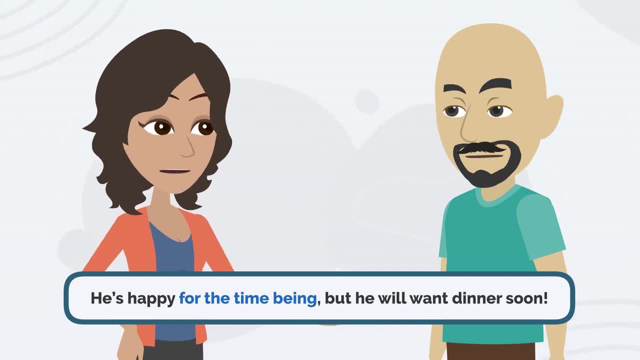 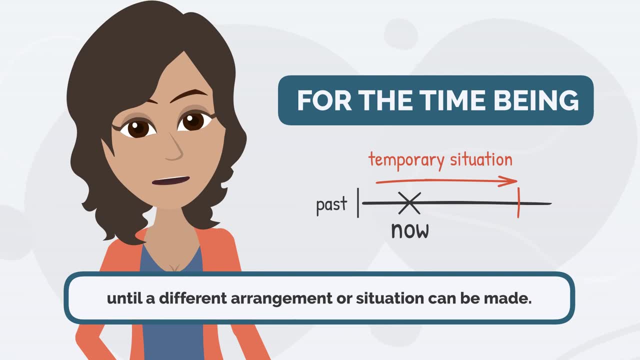 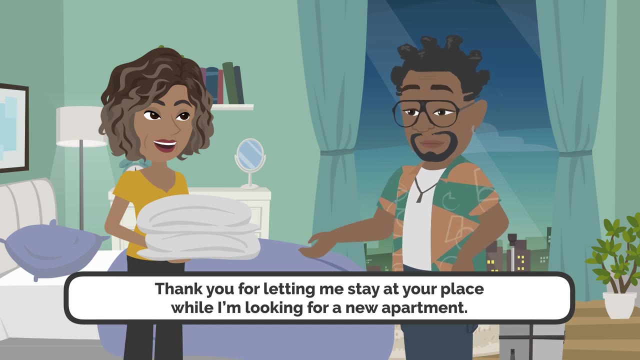 He's happy for the time being, but he will want dinner soon. For the time being means for a temporary amount of time until a different arrangement or situation can be made. Thank you for letting me stay at your place while I'm looking for a new apartment. 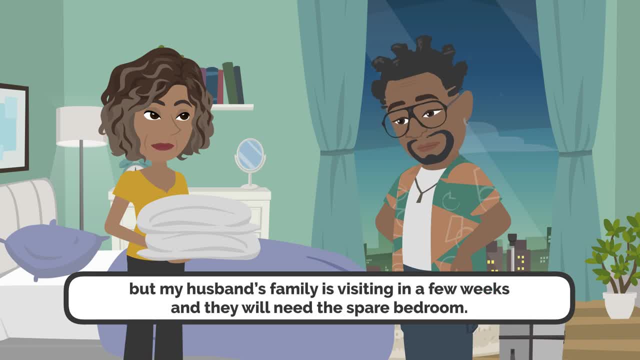 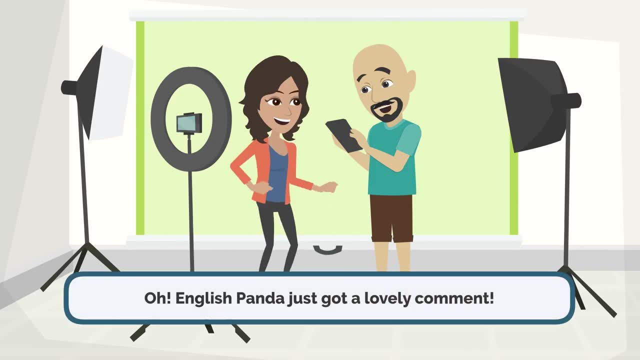 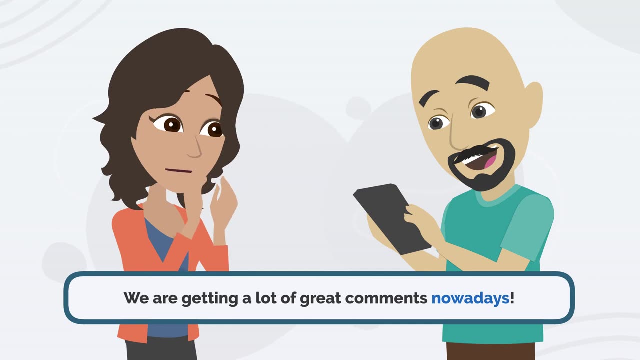 No problem, you can stay here for the time being, but my husband's family is visiting in a few weeks and they will need the spare bedroom. Oh, English Panda just got a lovely comment. We are getting a lot of great comments nowadays. 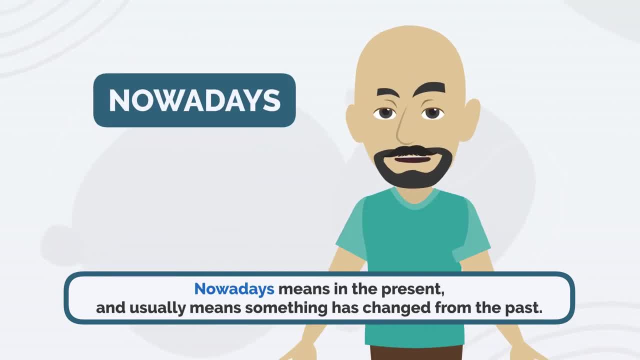 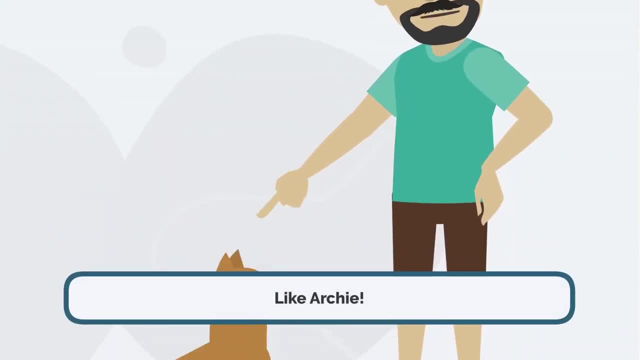 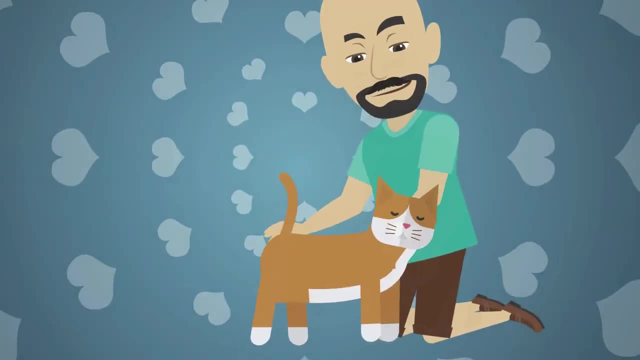 You're right. Nowadays means in the present and usually means something has changed from the past. Like Archie, He was very shy when we adopted him, but he is so cuddly nowadays. Meow, I love the way my humans have learned to follow my instructions. 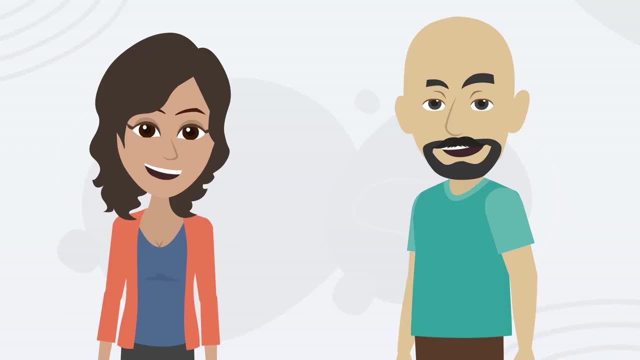 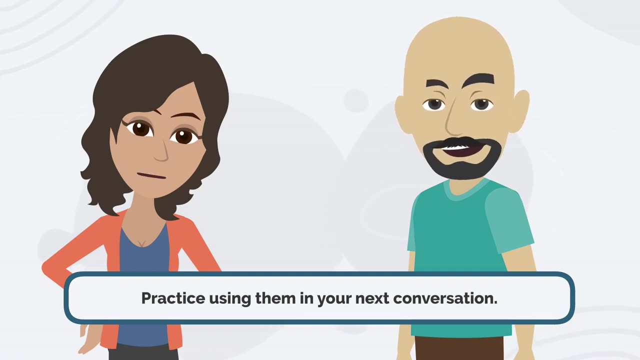 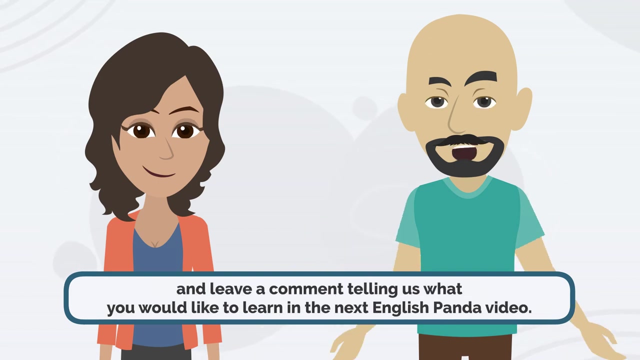 They listen so well. nowadays. These time expressions are all called common in English Practice. using them in your next conversation. Thanks for watching To let us know you've enjoyed this content. don't forget to like, subscribe and leave a comment telling us what you would like to learn in the next English Panda.